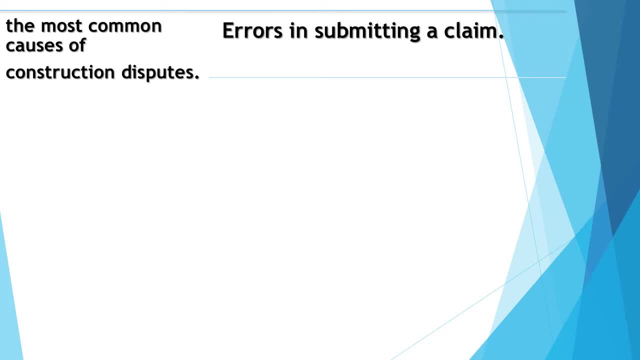 Poorly drafted claims without proper supporting documents can be grounds for disputes. Different site conditions: Bids are submitted based on current site conditions. This is why bidders are encouraged to visit the site before submitting their bids for evaluation. However, when construction begins, the condition of the site can vary due to soil condition, subsurface conditions and unexpected structures and obstructions. 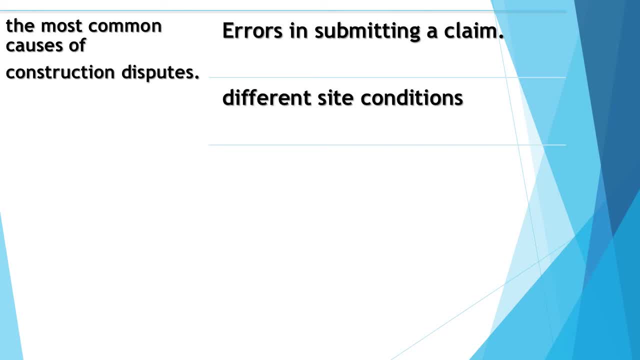 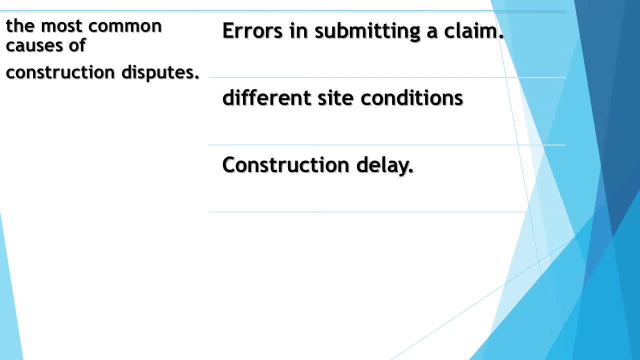 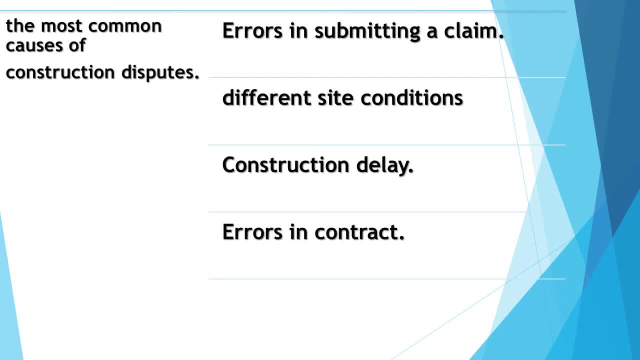 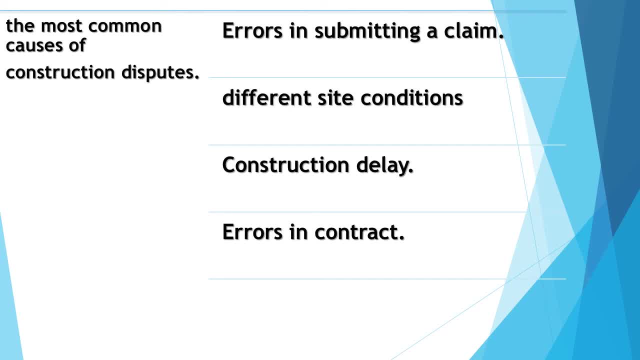 but with the right documentation and verification process, these mistakes are easy to avoid. the contract management process begins with a properly drafted contract document. if there are errors in the contract document, they can create grounds for disputes. many claim cases are not a good sign of contract management if the construction process does not comply. 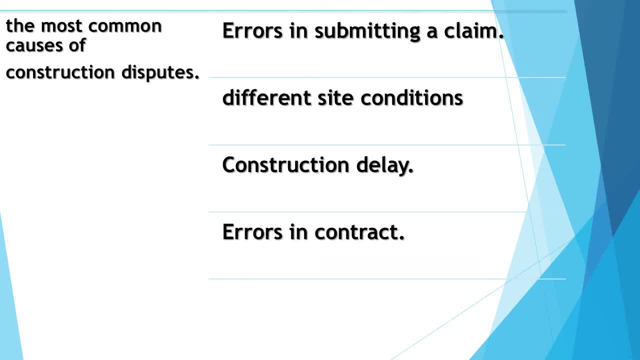 with the contract drawings and specifications. this is a cause of disputes. the contractor must follow the standards and specifications stipulated in the construction contract prior to delivery. defects and poor quality result in disputes between the parties not paying monthly invoices. the employer delays the payment of the specified time.